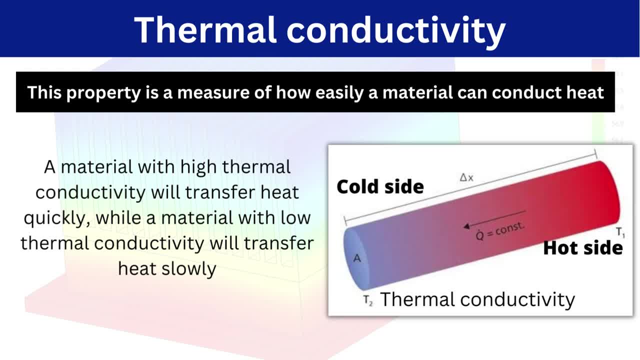 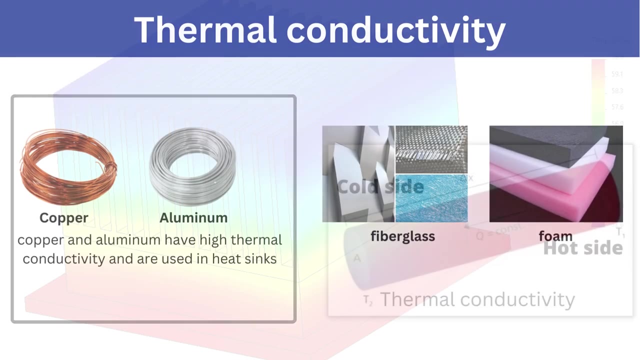 Okay means if at one end, suppose, the component is heated, so how easily the other end can be heat. Okay, because the heat is transferring. Okay, so the material with the high thermal conductivity will transfer the heat quickly and the material with the lower thermal conductivity will transfer heat slowly. Okay, and you can see the example. like copper and aluminum have the 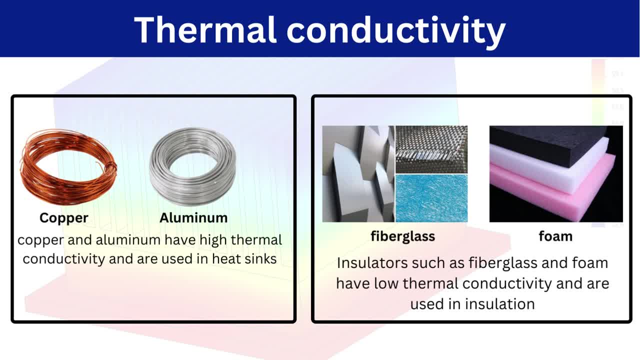 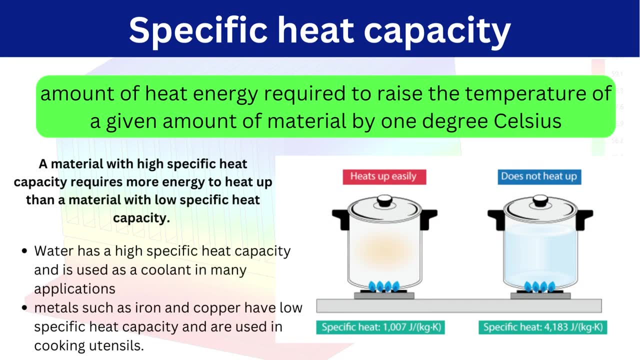 higher thermal conductivity and are used in the heat sink and the and the insulator, like fiberglass foam, have a lower thermal conductivity and are used in the insulation. So next one, we have the specific heat capacity. So specific heat capacity is nothing but the amount of heat energy required to raise the temperature of the given amount of material by one degree Celsius. 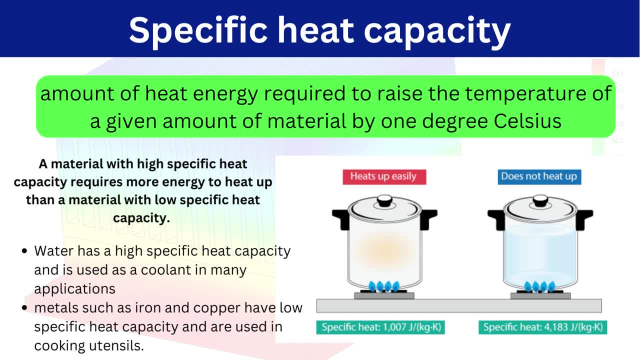 So the amount of energy required to raise the temperature to one degree Celsius is nothing but the specific heat capacity. Okay, so the material with a higher specific heat capacity required more energy to heat up. Then the material with a lower heat capacity. Suppose our material having the Have specific heat capacity. 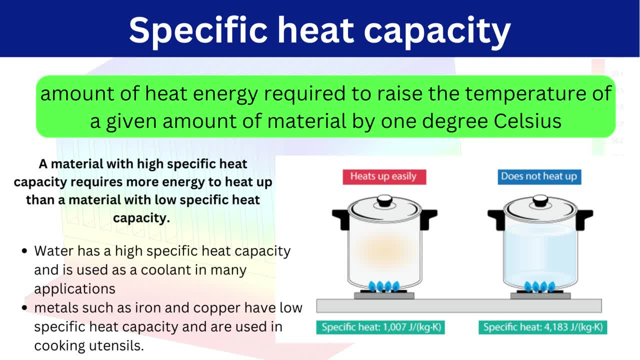 It means that we required the more energy or more heat to raise the temperature. so water has a high specific heat capacity and it is used as a coolant in many application. okay, because it required the uh- more energy or heat to raise the temperature. okay, while uh the metal, such as iron, copper, have the lower specific heat. 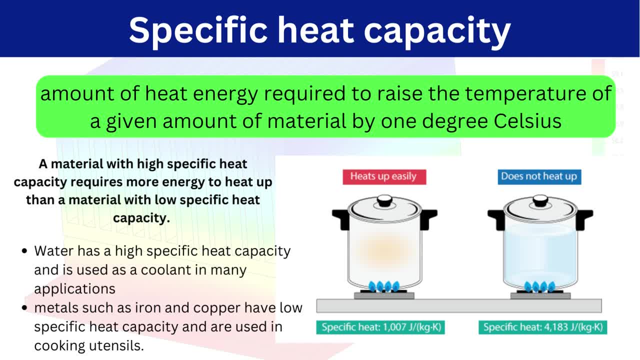 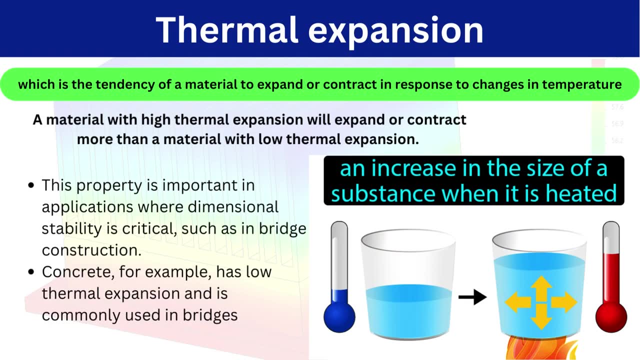 capacity and are using the cooking utensil, because in the cooking utensils we want the, we want the utensil easily heat up. okay, next one, we have the thermal expansion. so thermal expansion is nothing but the tendency of material to expand or contract in response to the change in the temperature. okay, so this property is 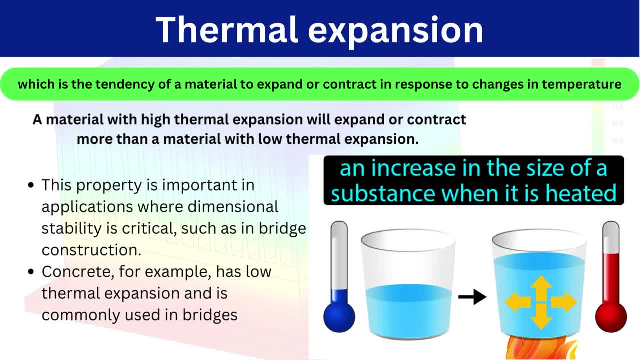 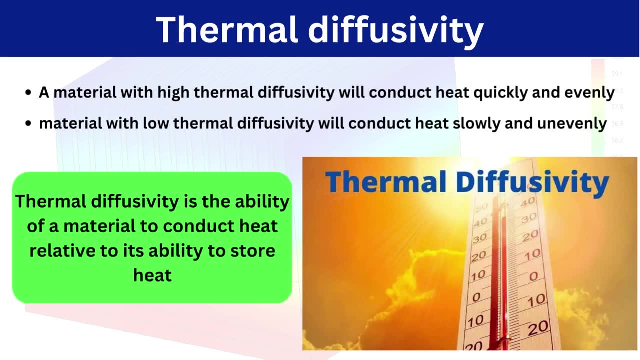 very important in application, where the dimensional stability is our requirement or the dimensional stability is critical at that time. thermal expansion properties very important. next one, we have the thermal diffusivity. so thermal diffusivity is nothing but the ability of material to conduct a heat relative to its ability to store the heat. okay, so the material 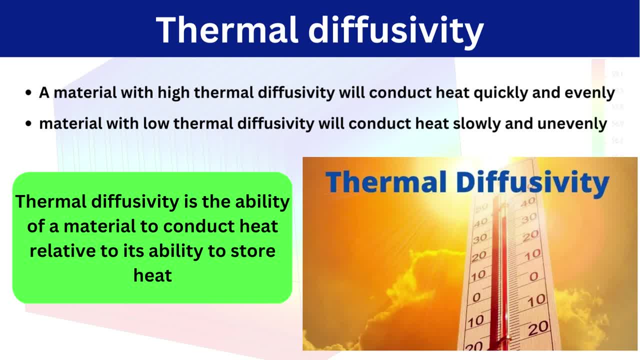 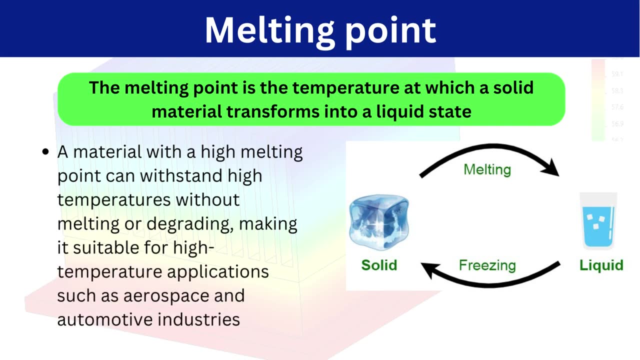 higher thermal diffusivity will conduct the heat quickly and evenly- okay, and the material with the lower thermal diffusivity will conduct the heat slowly and unevenly. next one: we have the melting point. okay, so the melting point, uh, is nothing but the temperature at which 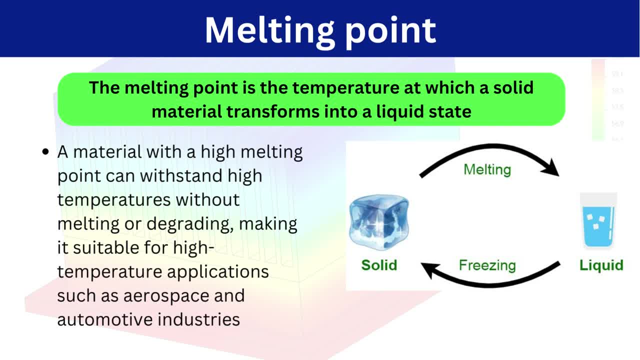 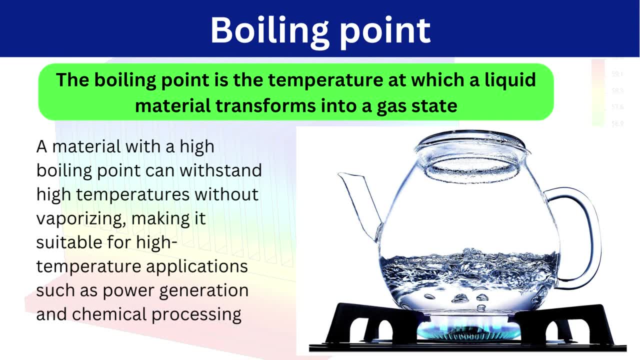 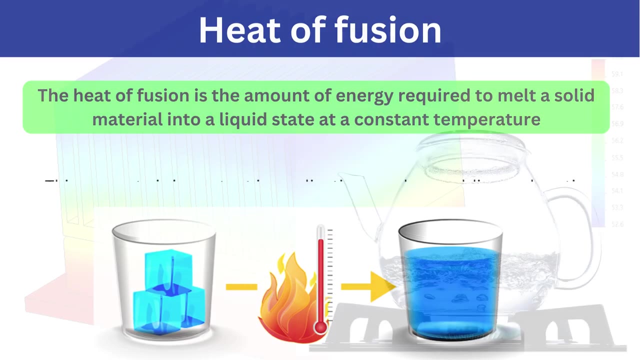 the solid state of material either transferred into the liquid state. next one: we have the boiling point. so the boiling point is nothing but the temperature at which the liquid state of material is transferred into the gas state. okay, so the material with a high boiling point can withstand the high temperature without vaporizing. next one: we have the heat of fusion. so the heat. 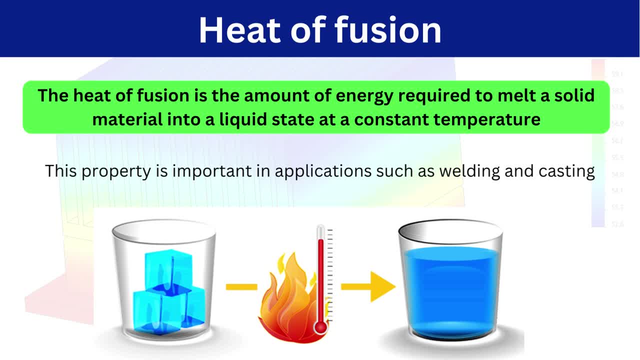 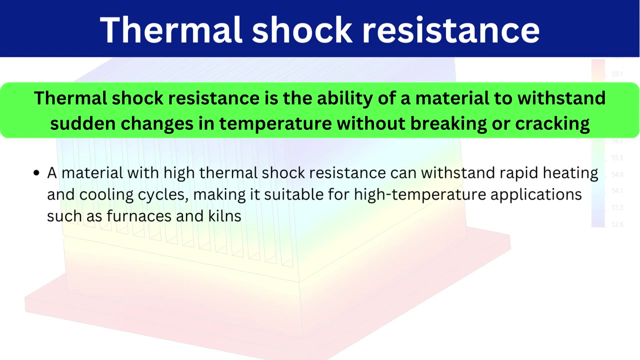 of fusion is the amount of energy required to melt the solid material into the liquid state at a temperature, so the heat of diffusion. this property is very important in application such as welding and the casting. next one: we have thermal shock resistance. so the thermal shock resistance is the property of material and is it is nothing but the ability of material to withstand. 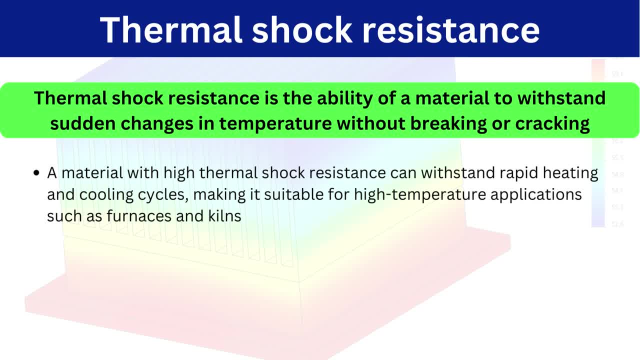 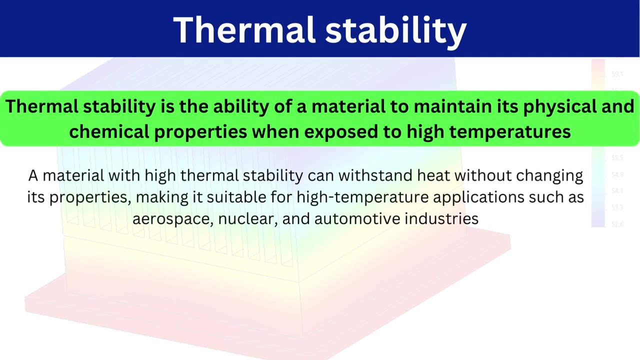 the sudden changes in the temperature without breaking and cracking. okay, so the material with the high thermal shock resistance can withstand the rapid heating and the cooling cycle. okay, so it is suitable for the high temperature applications such as the furnaces and the kilns. and the next one we have the thermal stability. okay so, the thermal stability.